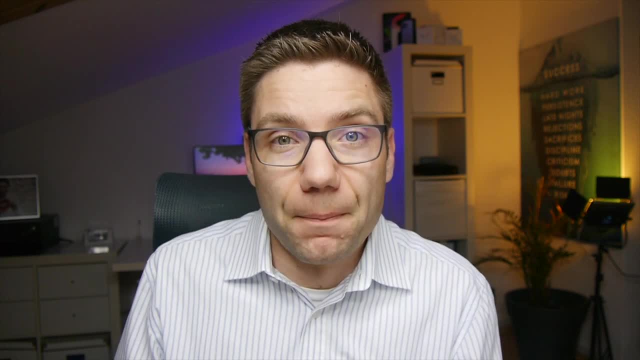 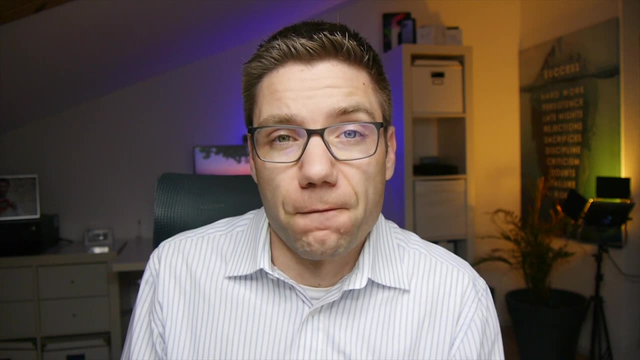 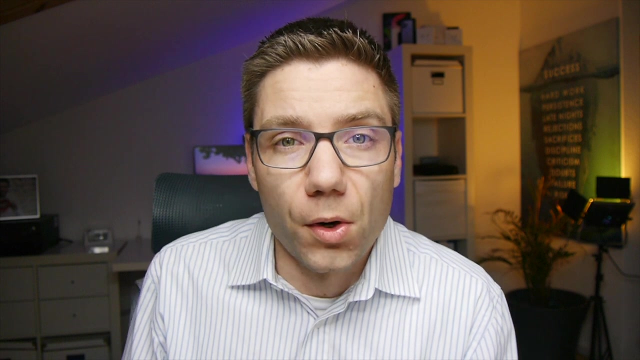 system is a computer system that is embedded into a mechanical or electronic system and is dedicated to a specific function. This could be, for instance, the microcontroller that is in your coffee machine, or it's the microcontroller that is in your light bulbs, and 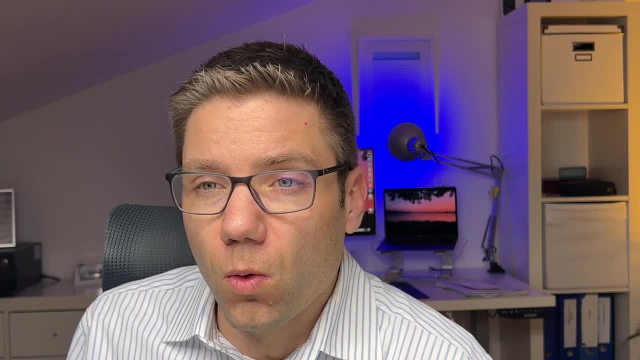 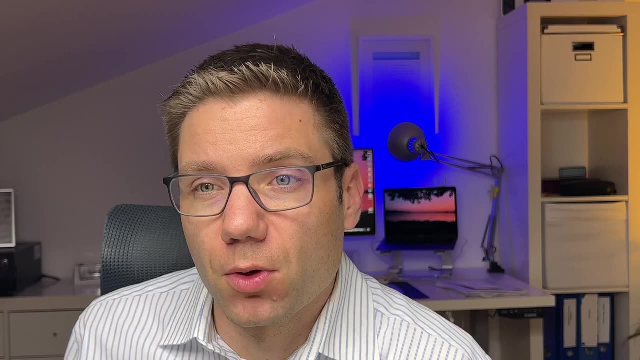 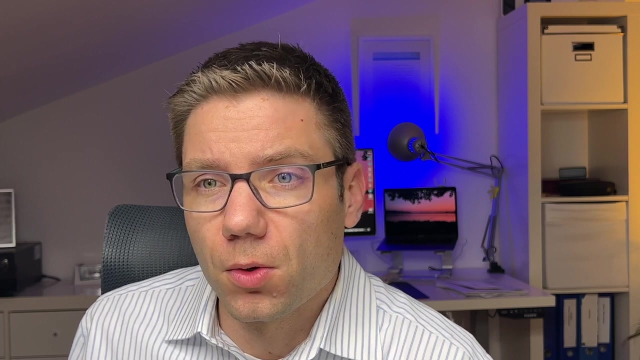 is able to change the RGB color, Or it's the control unit in your car that is protecting your life when you have a crash and is deploying the airbags, Or it's a flight controller in an aircraft Or similar things. It can even be an AirTag. 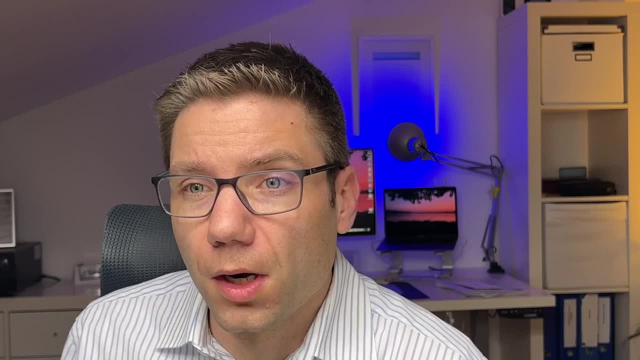 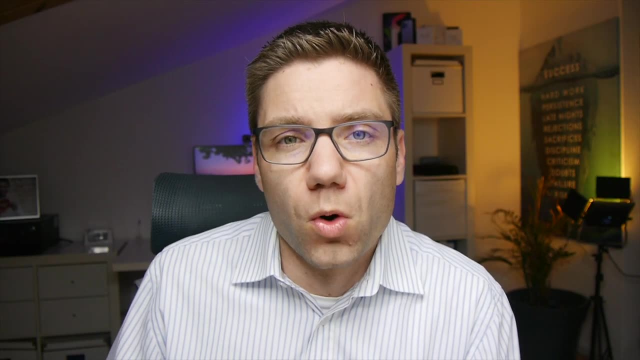 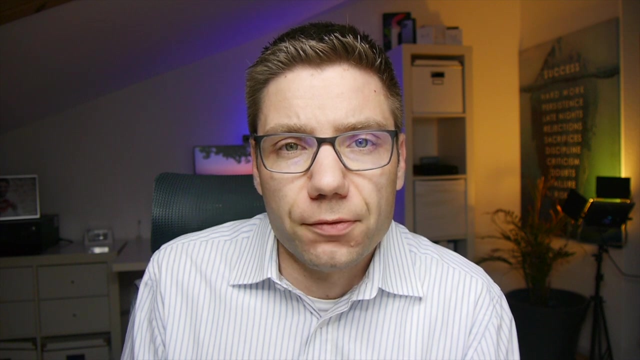 that is providing your position information, Or also in your airport, there is an embedded system. So what are the steps that you should take when you want to learn embedded systems and when you want to be an embedded engineer, Software engineer? The steps that I'm outlining here are not just, you know, a roadmap that I've 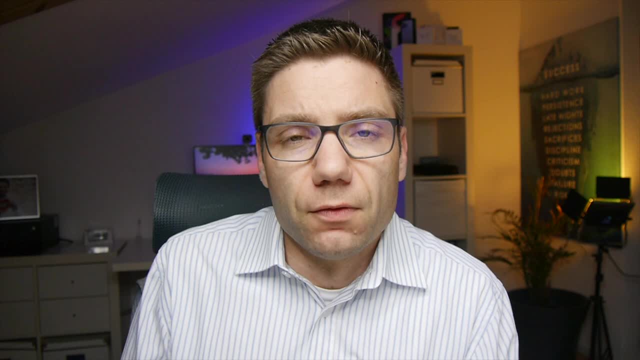 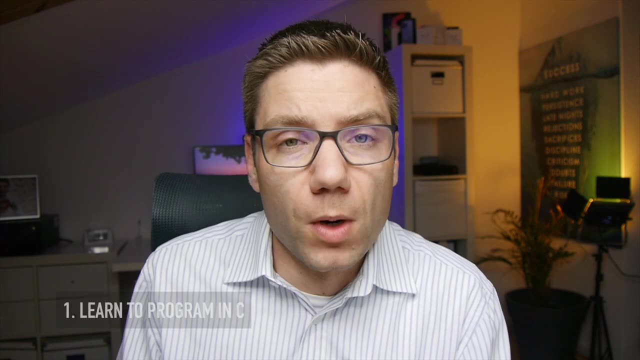 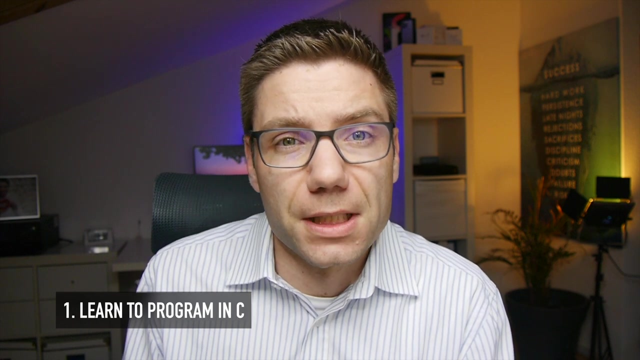 invented, but it's also the general theme that we use in our embedded systems program at the university. So let's start with step number one. Step number one is to learn the programming language C. There still is a lot of C used in embedded systems, even though there are 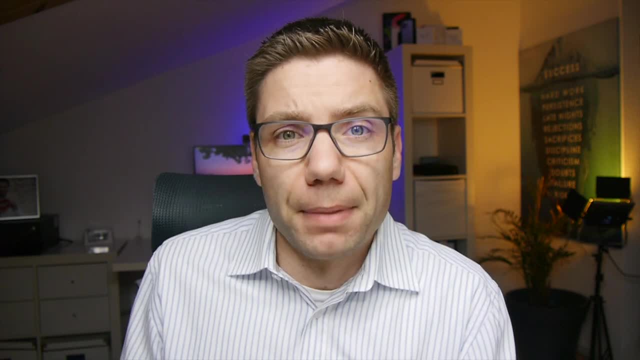 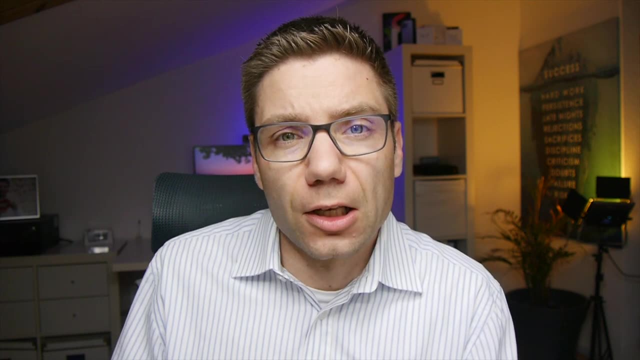 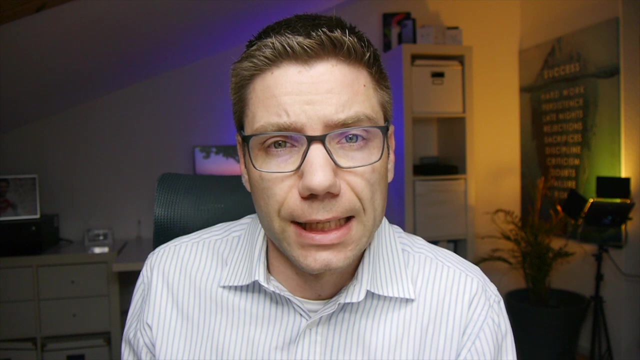 alternatives out there, like C++ and others, But C is actually the basic language that you can use. It's providing a lot of the foundations that you will later on need, even if you use a different language, like C++, And it gives you a lot of. 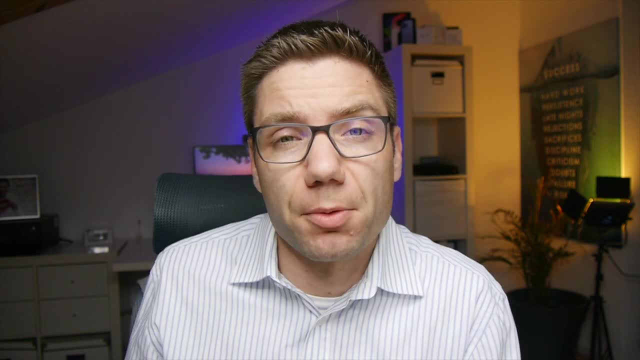 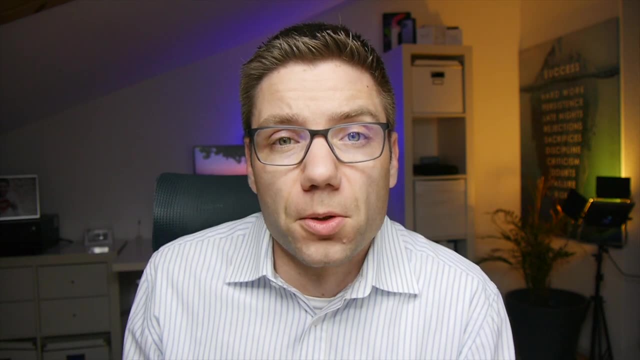 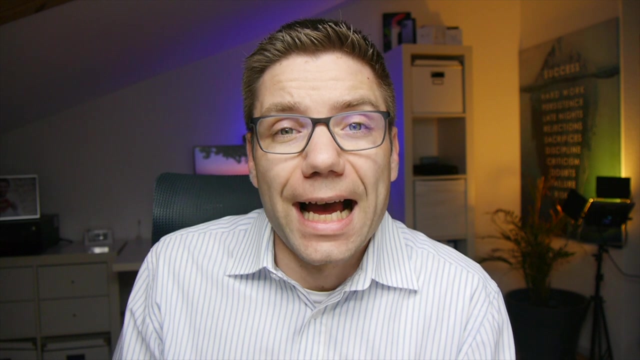 control over the microcontroller, over your embedded system, and it's very close to the actual hardware. The good news is you can even start learning C with your desktop computer, with system, with your windows environment. you don't have to start with an embedded system. i would 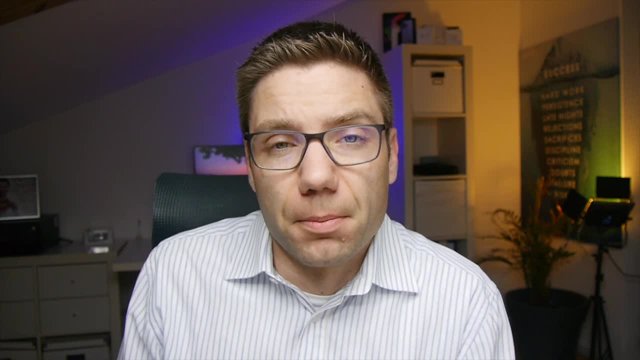 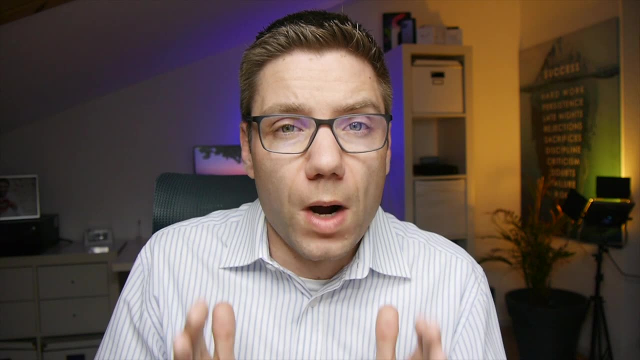 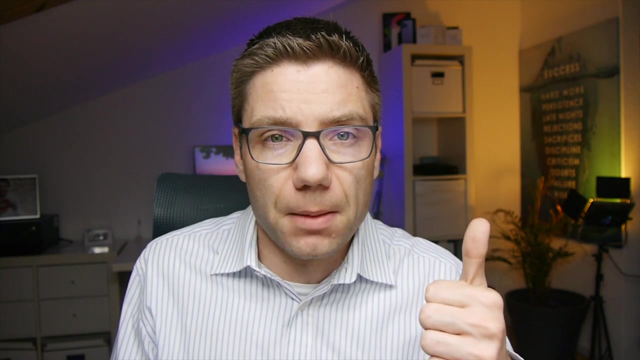 even encourage you to not start on an embedded system, start on your pc, start in your desktop environment, because then you can focus on learning one thing at a time, which is much easier than learning c and embedded systems at the same time. okay, so step number one: learn to code in c. step: 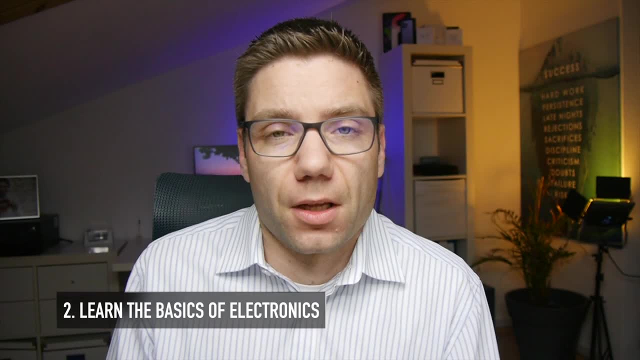 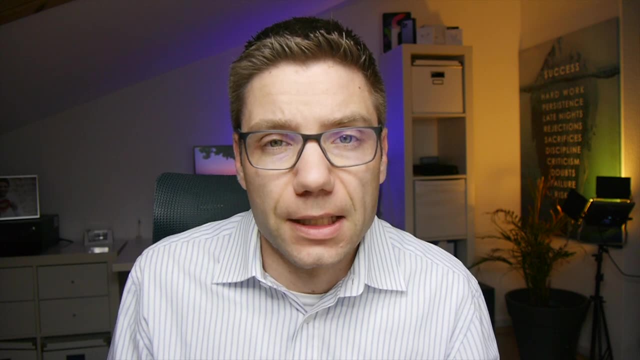 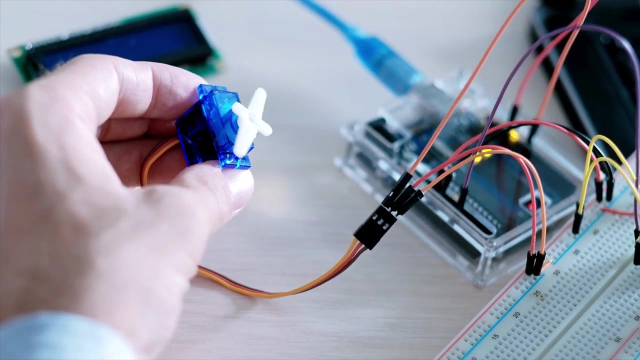 number two: learn the basics of electronics. when you deal with embedded systems, you are very close to hardware, so it's definitely a benefit to understand what a resistor is, to understand how an analog to digital converter works, what the limits are, what things you need to add to. 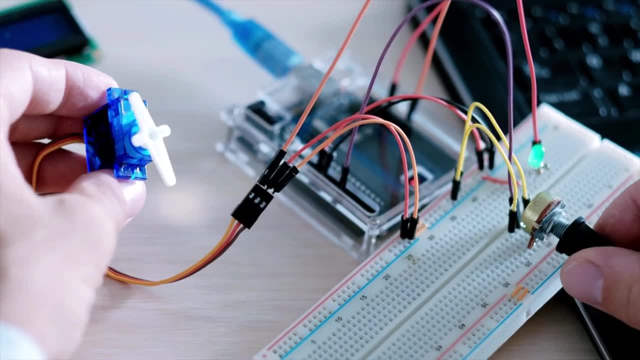 your microcontroller for a given project. so you need to have a basic understanding of the electronics to really learn how to code in c and embedded systems. so step number two: learn the basics of hardware. so you need to have a basic understanding of the electronics to really work. 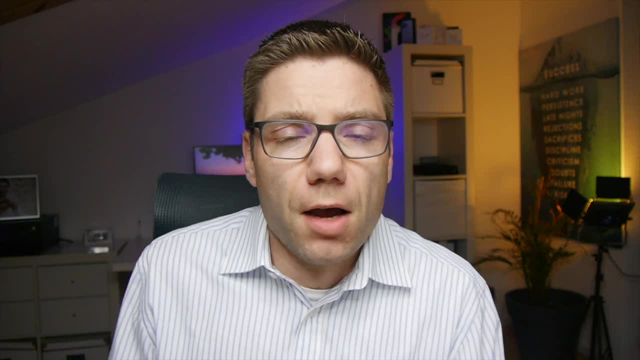 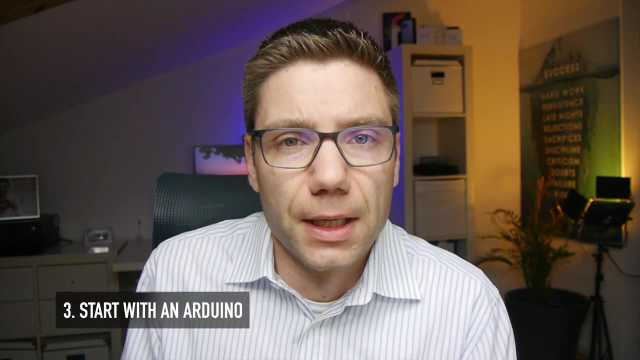 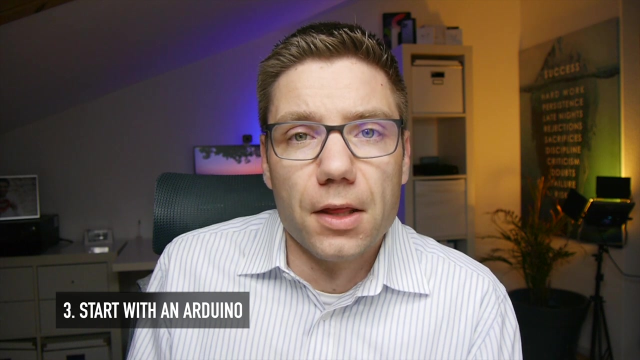 in the embedded systems field and then, once you have learned that the next step would be start with an arduino. the arduino system has two advantages that help you, as a beginner in the embedded systems field, to get started. the first one is it provides a lot of abstraction to the 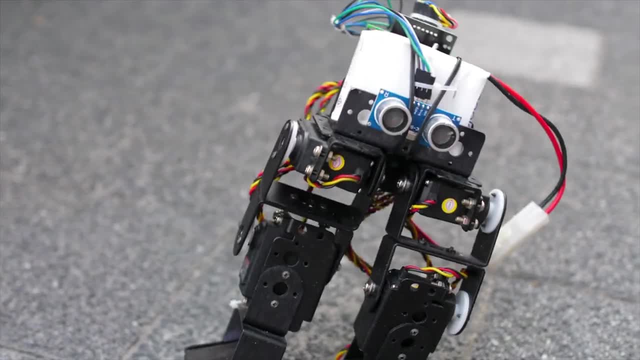 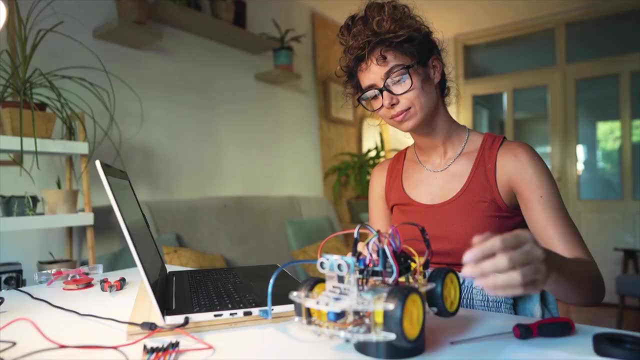 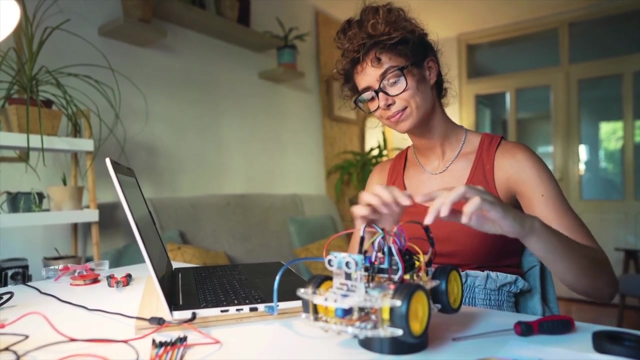 hardware functionality. so there are already a lot of libraries, a lot of things that come with an arduino system, that make it easier for you to work with the hardware, that make some of the things that are hard to do in c, in plain c, on a microcontroller, a little bit easier, and that's helpful especially. 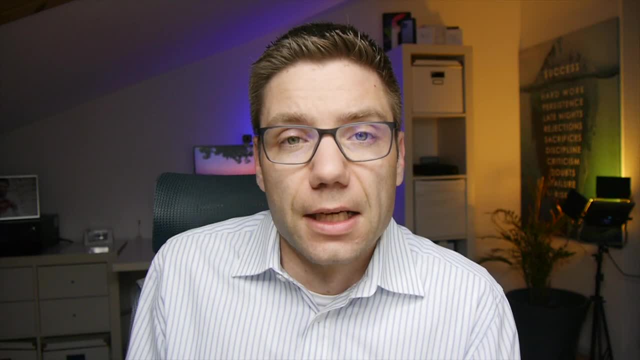 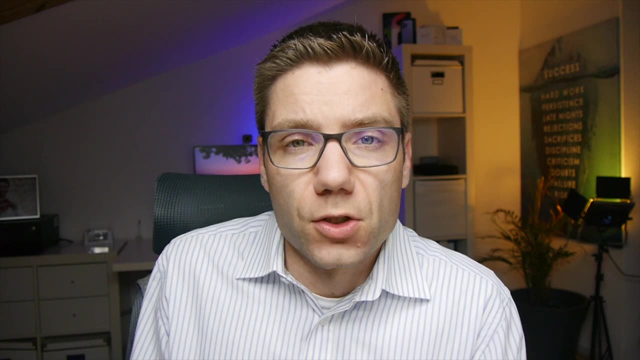 when you are a beginner. the second thing is there is very large arduino community and the community helps you in two ways. the first one is you will always find project ideas. you will always find showcases of projects and you will always find project ideas and you will always find. 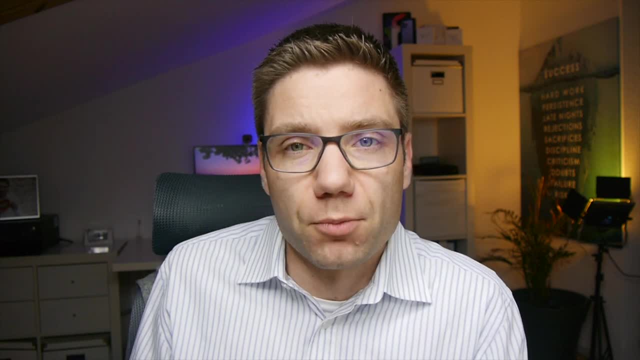 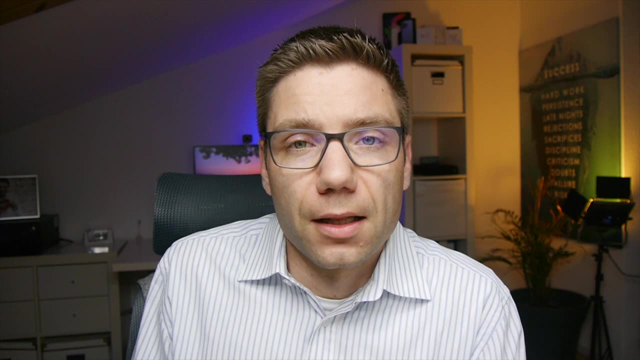 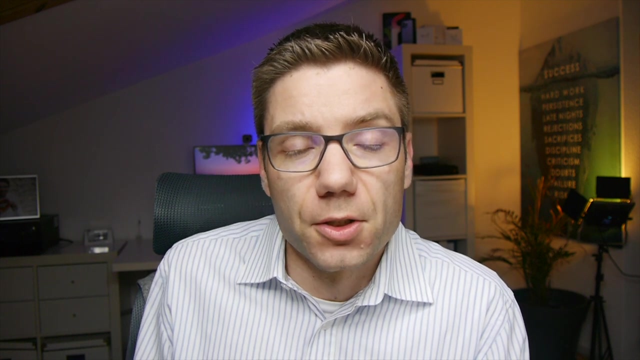 also find the kits that you need that provide all the different electronic parts for this project. and the second thing is, there is a very large community and that's, of course, helpful whenever you have a problem, because chances are, you're not the first one that has this problem and the 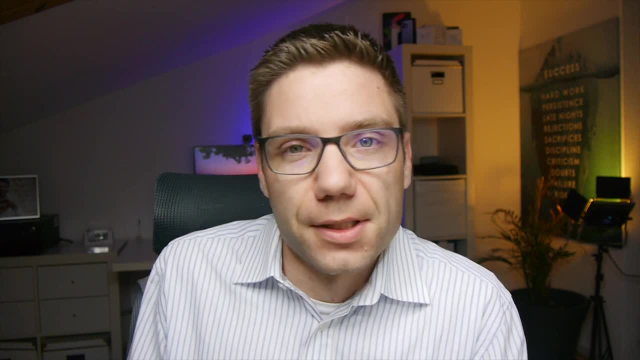 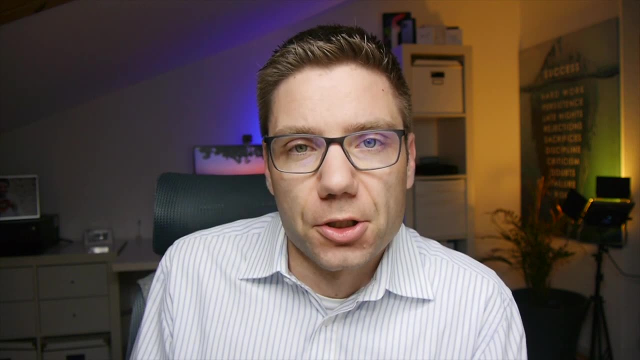 questions have already been asked and answered on Stack Overflow or similar websites, so that's a big plus. if you start with something likechanticecom link in the description or in the user label has a large community number. four would then be taking this to the next step once you feel. 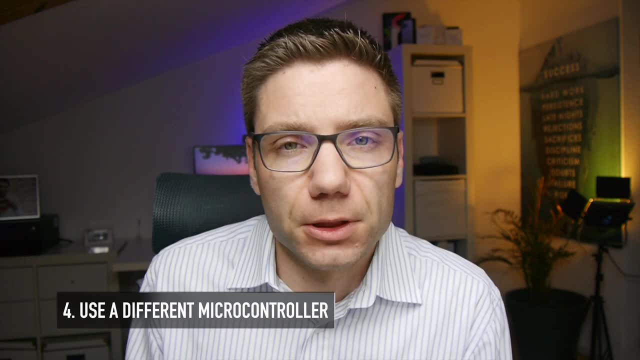 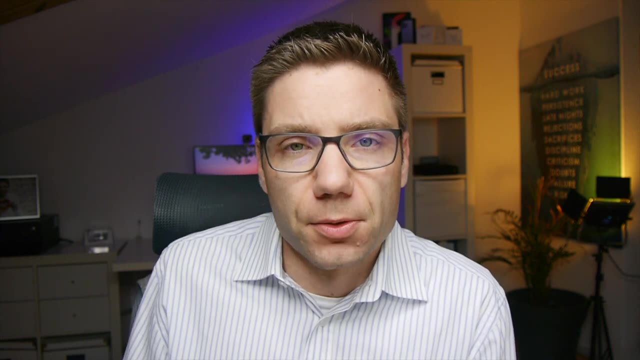 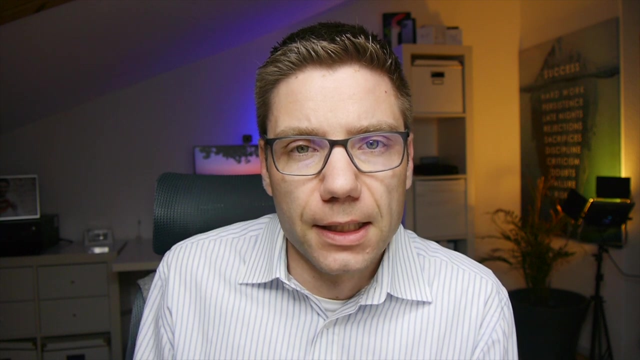 confident with the arduino. once you feel comfortable with the arduino, take the step to a more barebone microcontroller. for instance, you can use the st nucleo boards that provide you a more microcontroller like feeling, which means you have more control over the microcontroller. 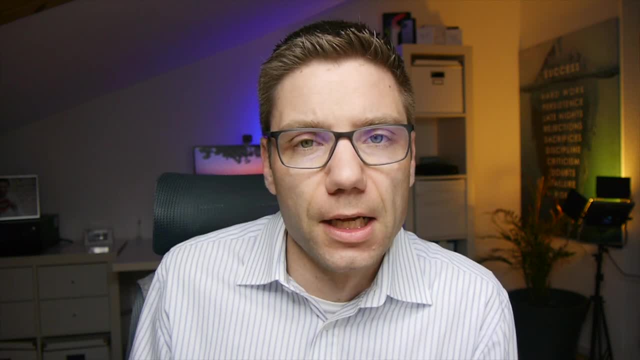 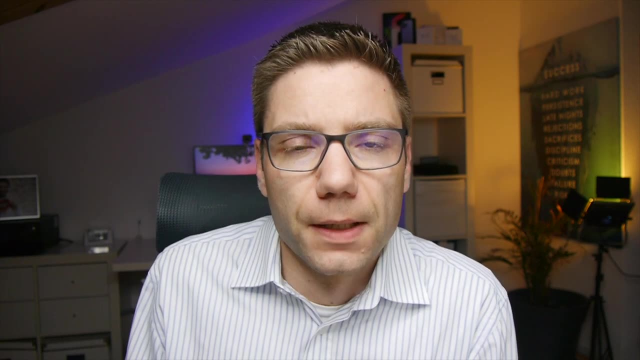 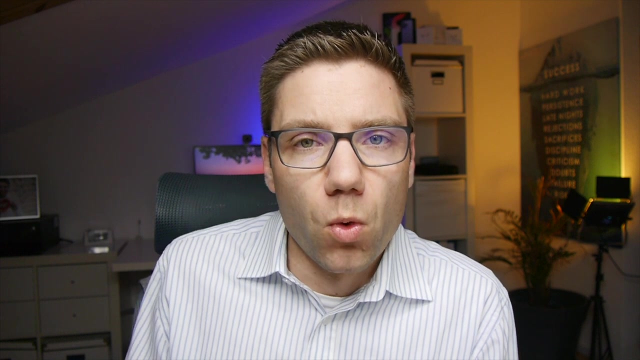 you have less libraries that are already there and are sort of restricting the access that you have to the microcontroller. you get a full-fledged jtech debugger port and things like that. so you have more control but of course, on the other hand, also more code that you have to write. you get the. 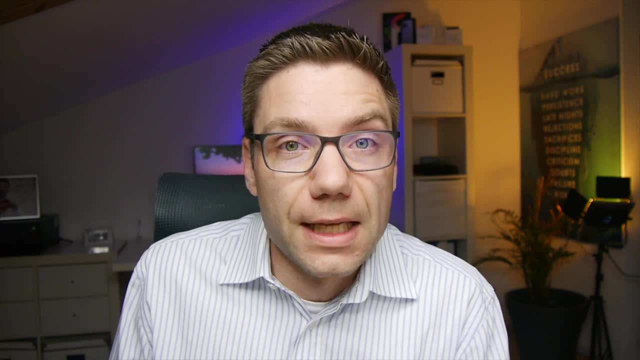 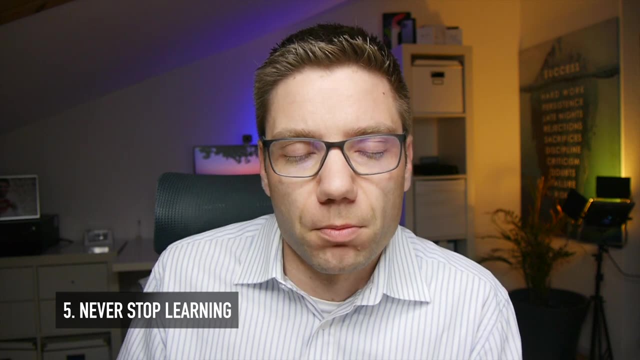 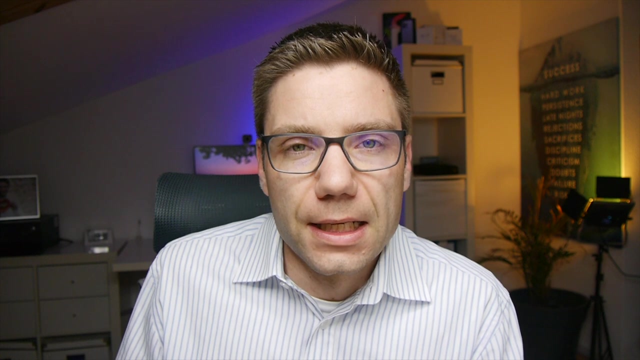 board running to get your projects running. and then the fifth step is never stop learning, right. you might have built several projects with arduino already. you maybe have built your first or second project with the st nucleo board or similar boards, and then really it is about going from project to project, increasing the complexity, increasing. 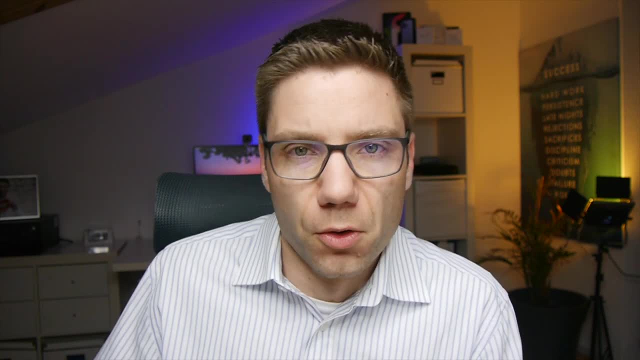 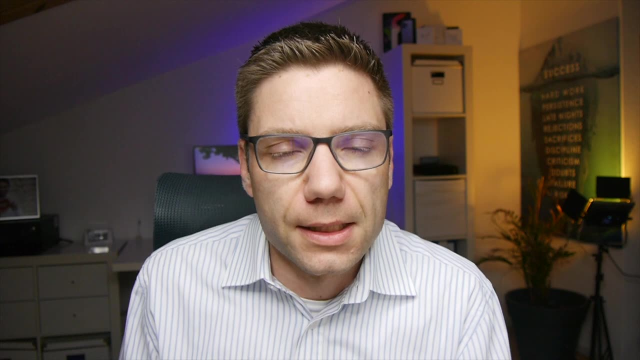 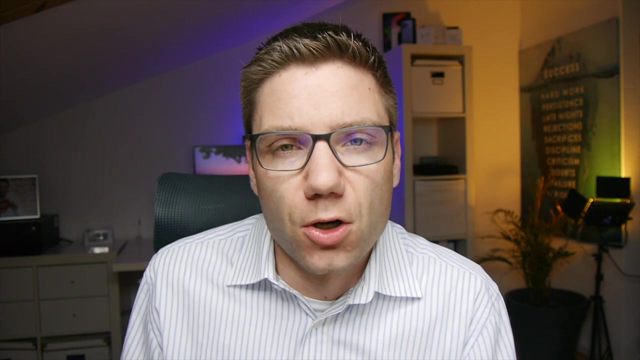 the difficulty of the projects and to learn, learn, learn, learn and master the art of embedded software engineering. so you will see, there are a lot of great things that you can build with embedded systems. there are a lot of very exciting projects, whether that's home automation, whether that's building a self-driving car, whether that's. 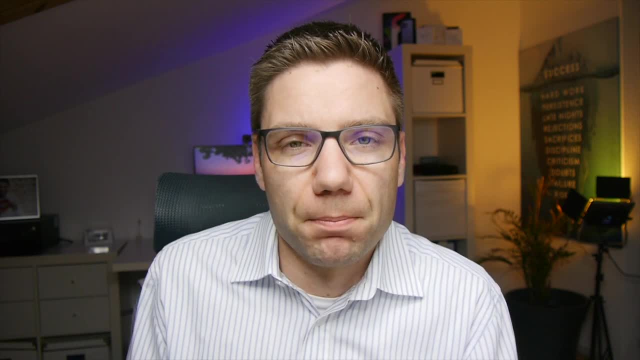 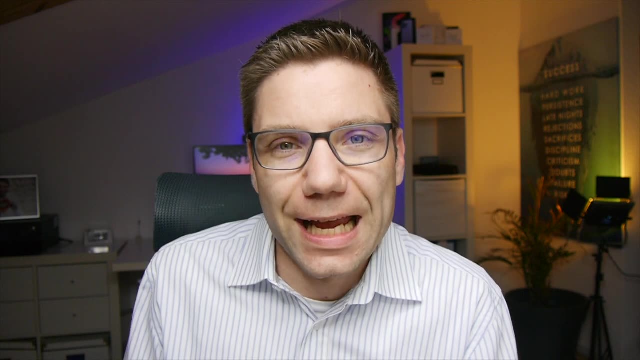 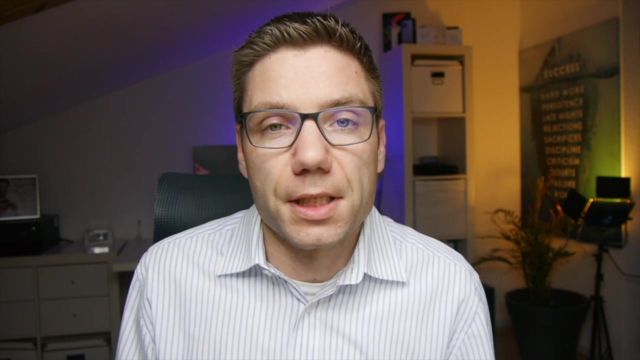 robotics. there are a lot of very nice things that you can build with embedded systems, and it's really something that's worthwhile learning and very, very interesting and a lot of fun. so, for all the five steps, i will create a list of resources that i can recommend for those specific. 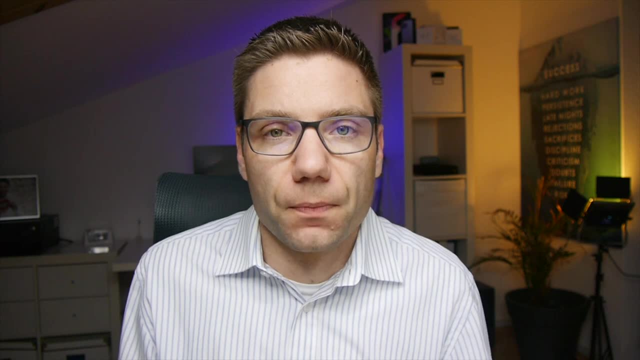 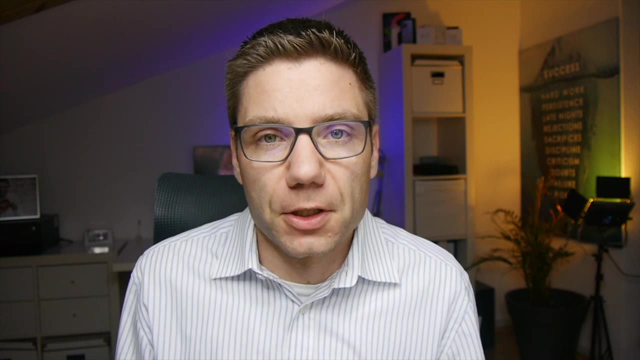 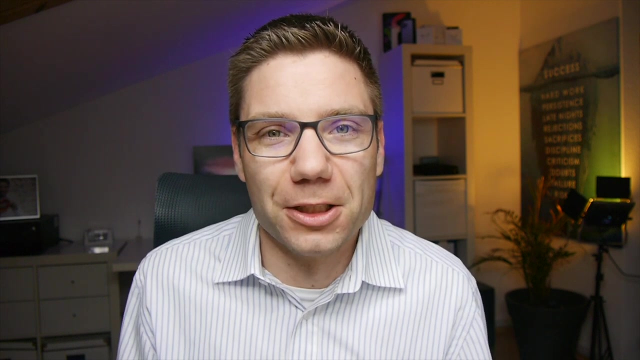 steps. you will find the link in the description box below and i will also put a link to the link to this list in the description of this video. i will also update this list from time to time if something changes and i'm sure you will have a lot of fun exploring embedded systems building.